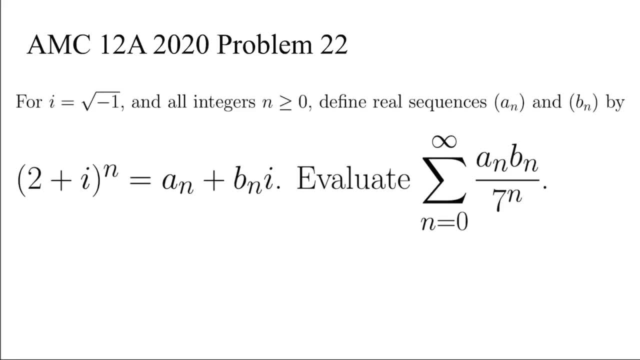 Let's take a look at this problem taken from the American Mathematics Competition, AMC12.. For i equals the square root of minus 1, and for all integers n that are non-negative define real sequences: a, n and b n by 2 plus i to the n equals a n plus b n times i. 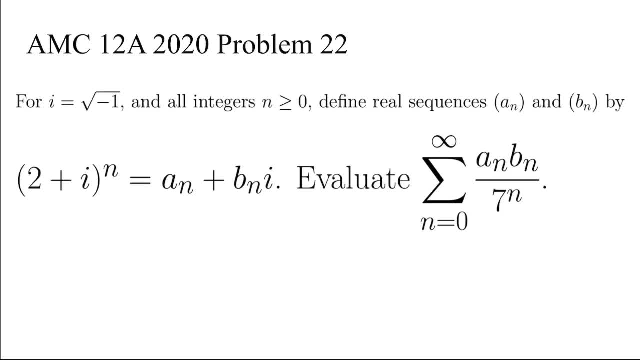 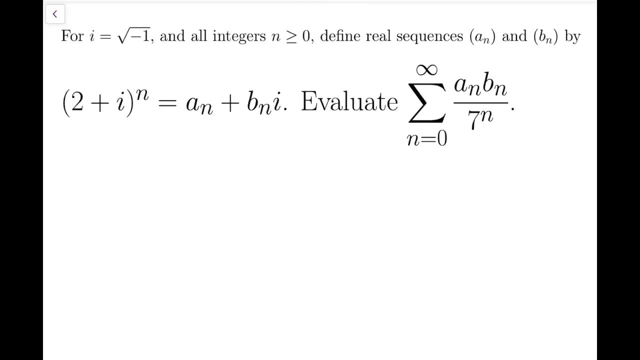 Evaluate the sum of a, n, b, n over 7 to the power of n, from n equals 0 to infinity. Before we move on, don't forget to give a like, subscribe to my channel and turn on post notifications. In this video, we are going to learn how to divide real and imaginary parts into a polar form. 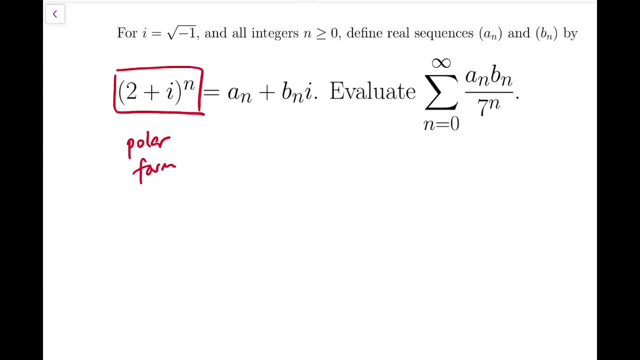 The so-called polar form is similar to polar coordinates and it is about the magnitude of the modulus and the angle of the line between the polar coordinates and the imaginary coordinates. Evaluate the thing of the line 2 plus i. that represents 2 plus i. 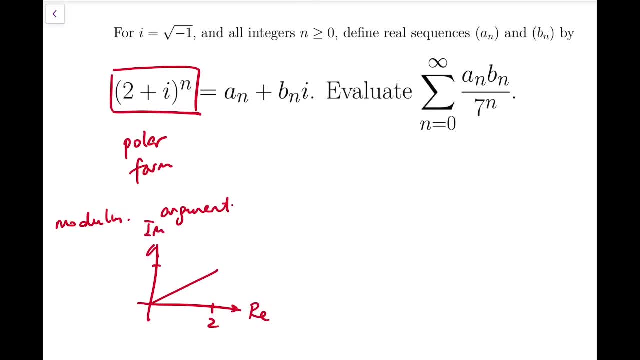 say it's 2 for the real part and 1 for the imaginary part. Here is 2 plus i, and we consider the angle instead. So this is the modulus, which is in fact equal to square root of 2 square plus 1 square. 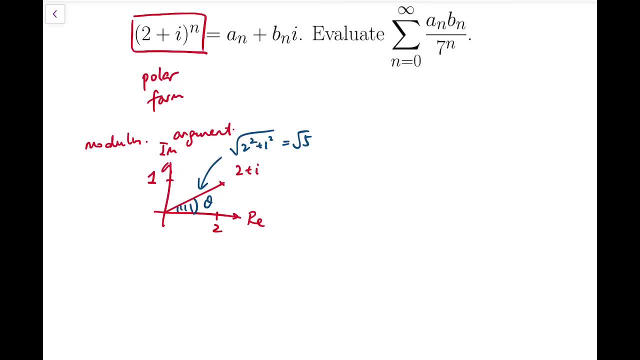 equals square root of 5.. And then here is An angle, which is the argument defined by tangent: theta equals a half. Similarly, we can deduce that sine theta is 1 over square root of 5, Cos theta is 2 over square root of 5. 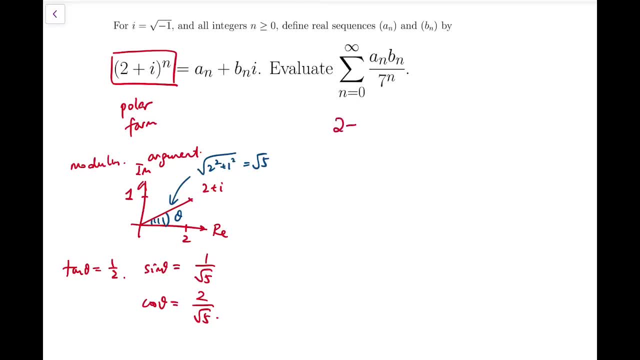 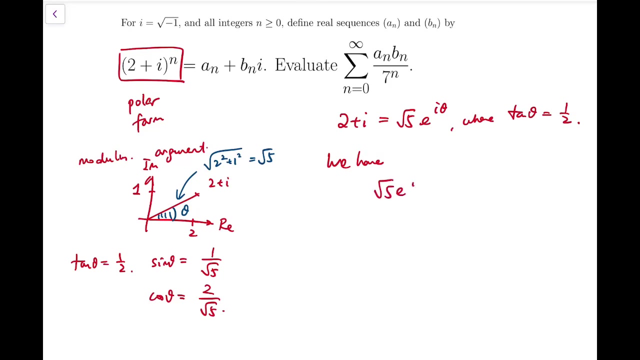 So that's about the polar form. Now 2 plus i can be written as root 5, which is the modulus times e to the i theta, Where tangent theta equals a half, And by rewriting this we have Root 5. e to the i theta whole thing to the power n. 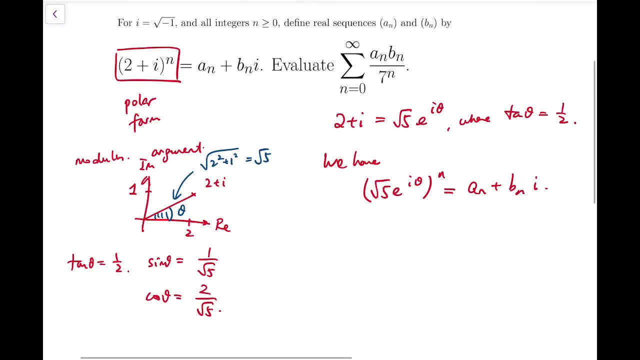 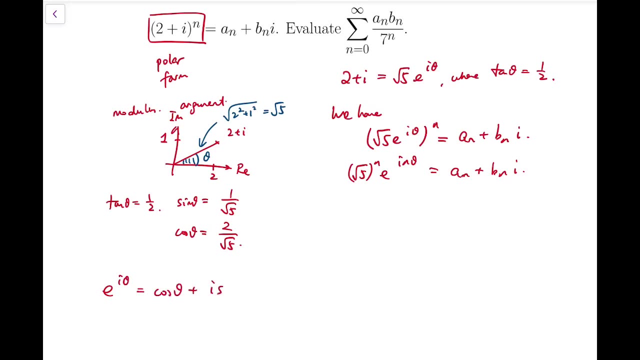 Equals a n plus b n i, And so root 5 to the n, e to the i? n theta equals a n plus b? n. Here we define e to the i theta by cos theta plus i sine theta, And so by comparing real and imaginary parts, we can say that 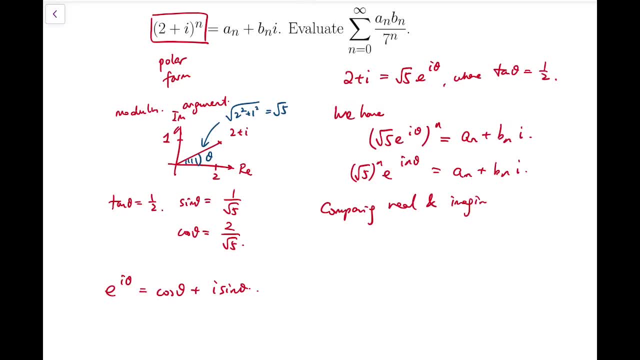 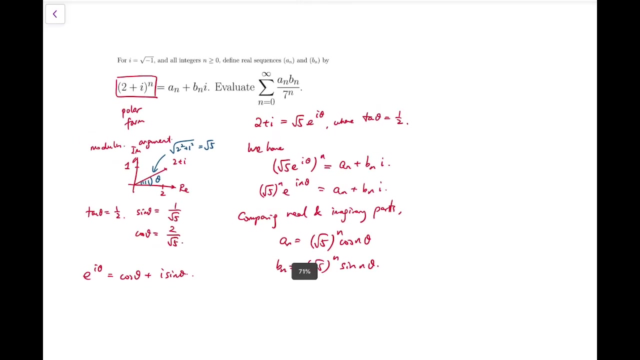 a- n equals square root of 5 whole to the power n Cos n theta, and b? n e to the i theta Equals something similar but sine n theta instead. Now we have successfully written a? n and b? n into some very condensed form, So we can now turn to evaluate that sum instead. 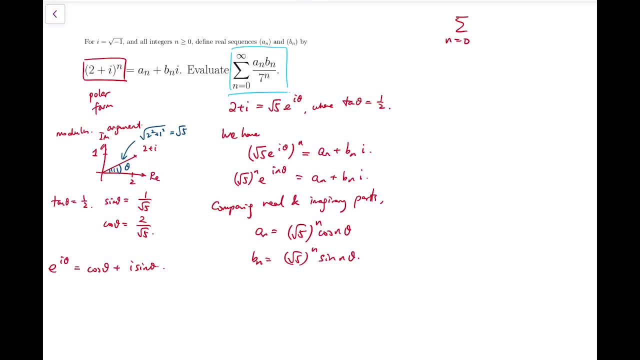 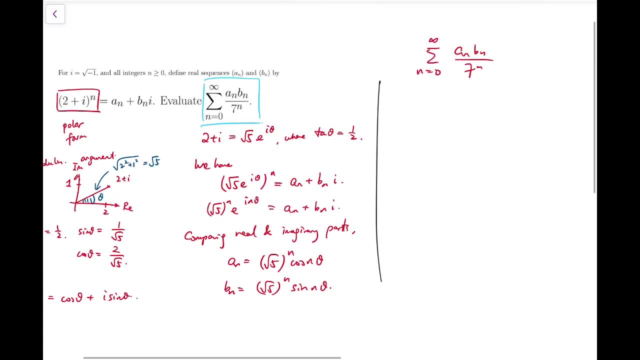 So this sum Now becomes The sine of 2 theta is actually 2 times sine theta cos theta. So this matches what we have at the moment. So that's actually equals to a half Times sine 2 n theta. Now, at this stage we can actually make use of the polar form again. 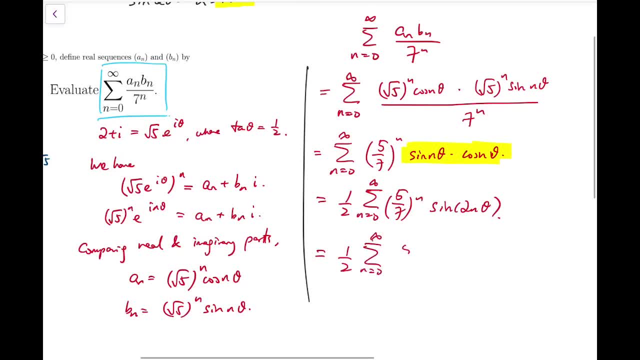 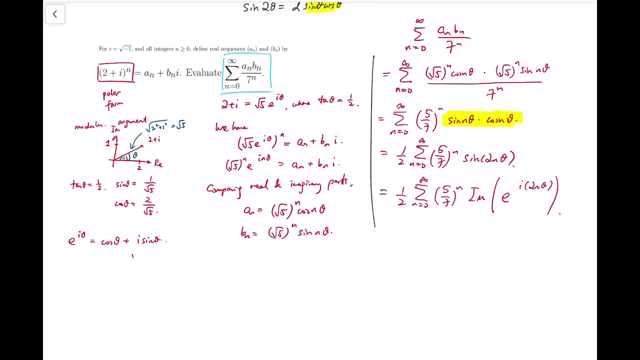 And rewrite the sine term As the imaginary part, Imaginary part, of e to the i times 2 n theta. Now, from this definition, e to the i theta equals cos plus i sine. We can say this As cos of 2 n theta plus i times sine of 2 n theta. 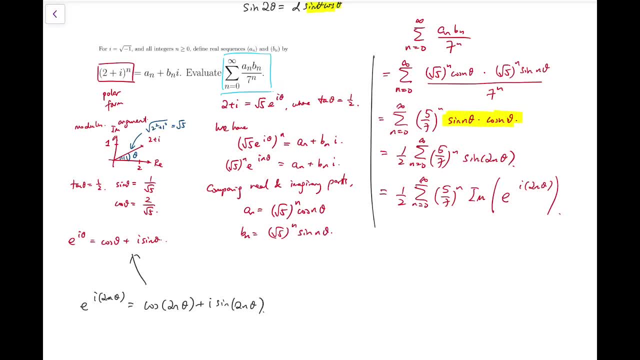 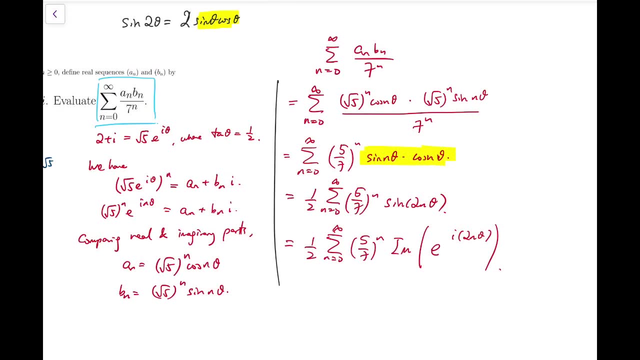 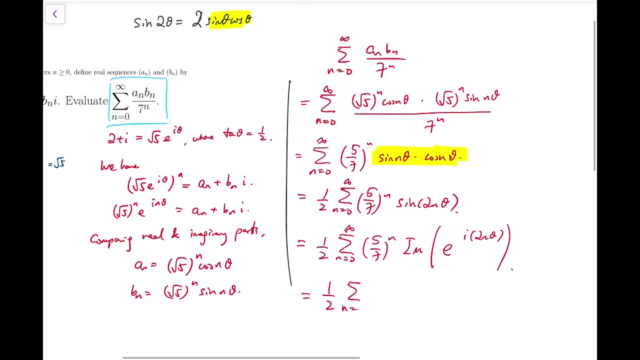 So sine of 2 n theta equals sine of 2 n theta. The sine 2 n theta is exactly The imaginary part of e to the i times 2 n theta. Now with this I can put everything into the imaginary part bracket By saying: 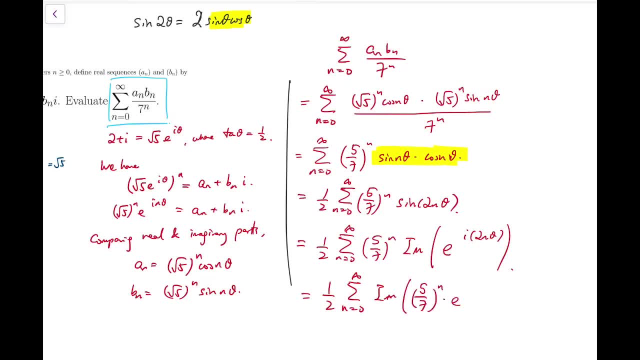 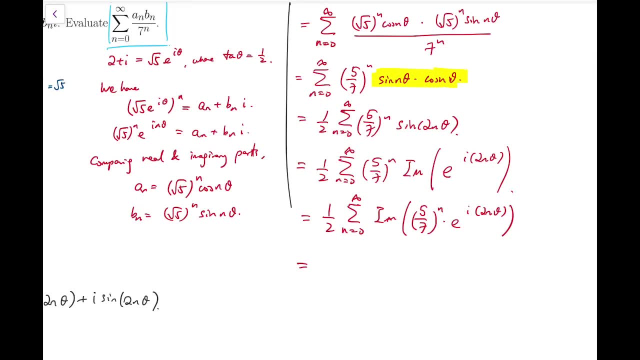 It is the imaginary part of 5 over 7, to the power n times e, to the i times 2, n theta, and similarly, because the sum of the imaginary parts of the complex numbers are actually equal to the imaginary part of the sum. So we can kind of swap the sequence, swap the operation sequence. 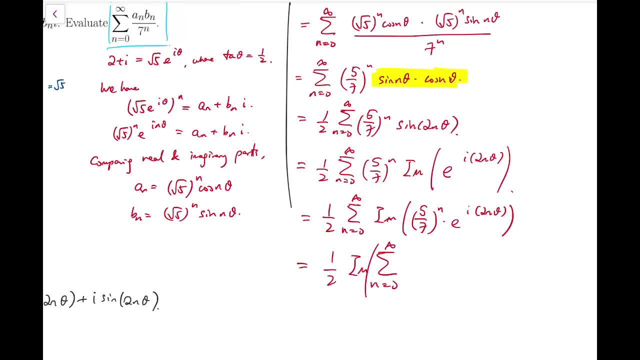 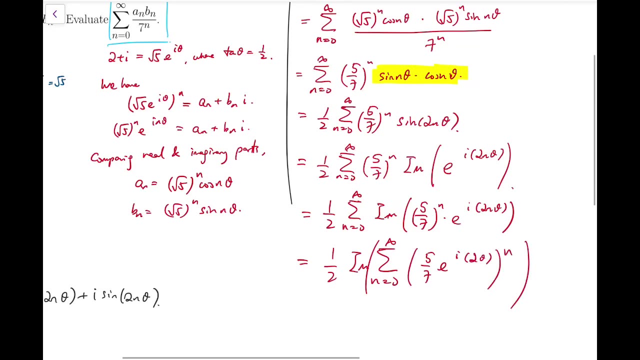 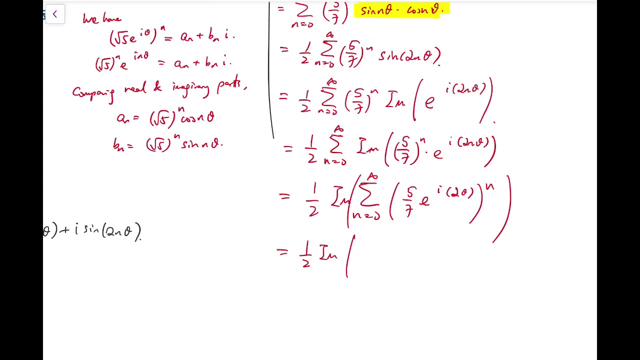 So I can swap the signs And rewrite this into: 5 over 7 times e to the, i times 2 theta and the whole thing to the power n. Now the sum inside labeled with green is actually equal to the sum of the imaginary parts of the complex numbers. 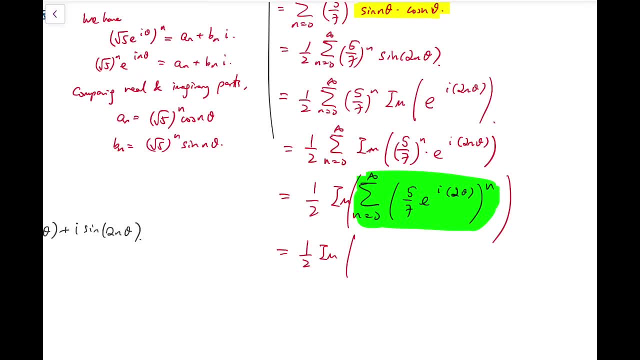 So we can kind of swap the sequence, So we can actually do a geometric series with a modulus that is between minus 1 and 1, because the term inside 5 over 7 times the e power actually has modulus 5 over 7.. 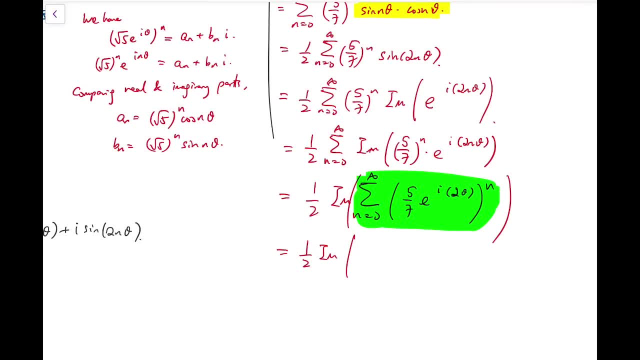 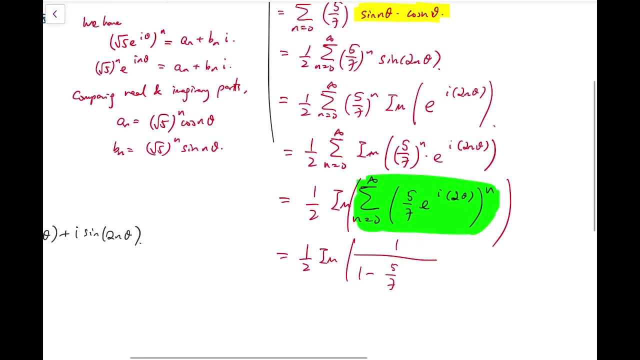 So I can apply the infinite series formula, which is the first term, is just 1, because the zero power is 1.. And then the common ratio is 5 over 7.. 5 over 7 times e to the i times 2 theta. 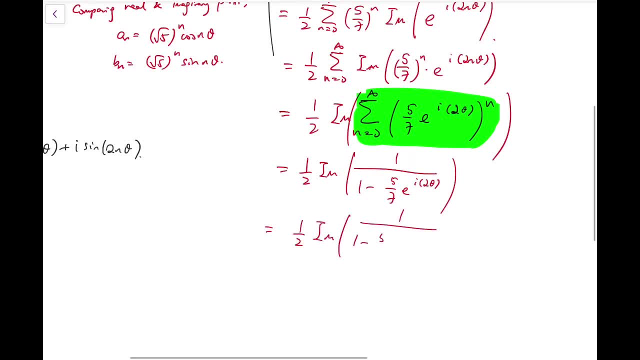 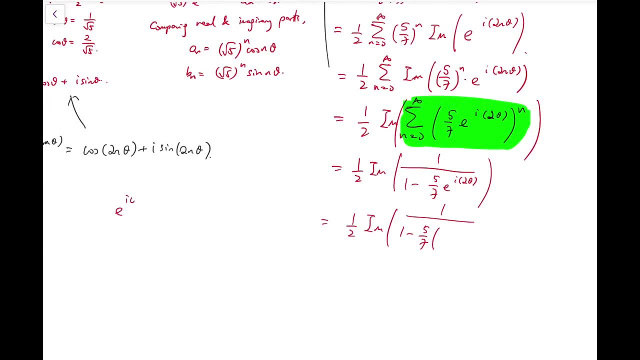 So 5 over 7 times. now we have to calculate e to the i times 2 theta. Now we know that e to the i theta is just 2 plus i. So e to the i times 2 theta, It's a square.